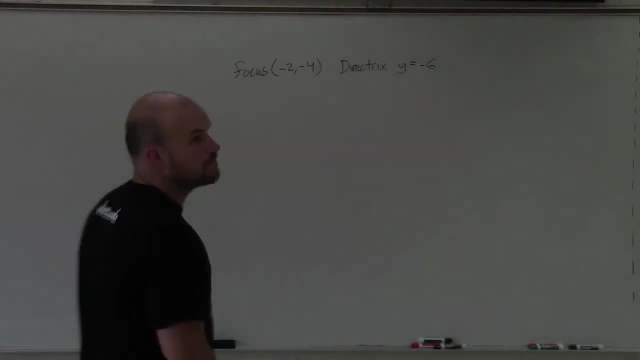 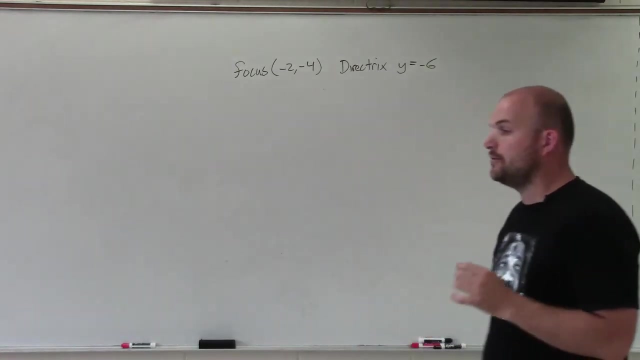 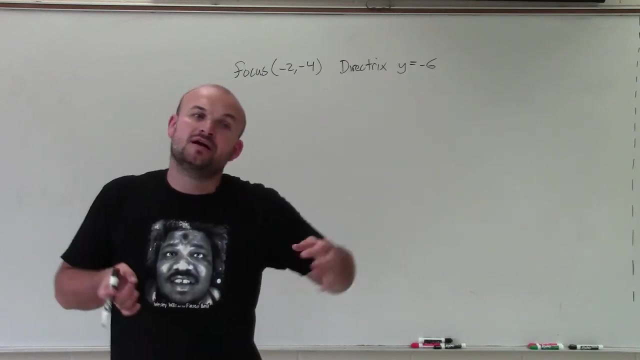 Welcome, ladies and gentlemen. So what I'd like to do is show you how to write the equation of a parabola, given the focus and the directrix. Now remember the definition of a parabola, using our conic sections, is the distance from any point on a parabola to the focus. 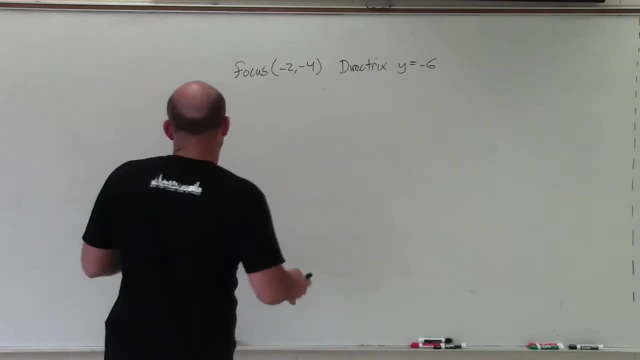 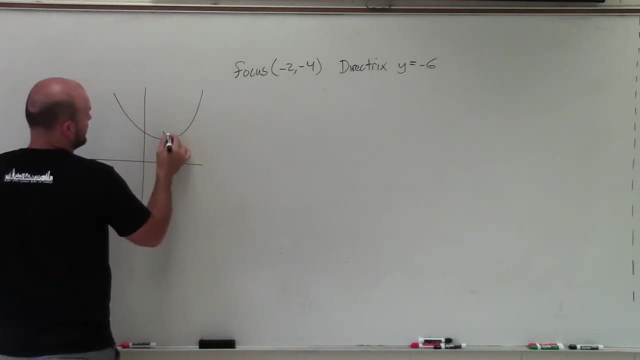 and the directrix is equal. Now, the most important point that I would probably say on a parabola that we'd want to be looking at would be the vertex, And let's say I have a vertex here And let's say the focus is right there. Well, this directrix, the distance, 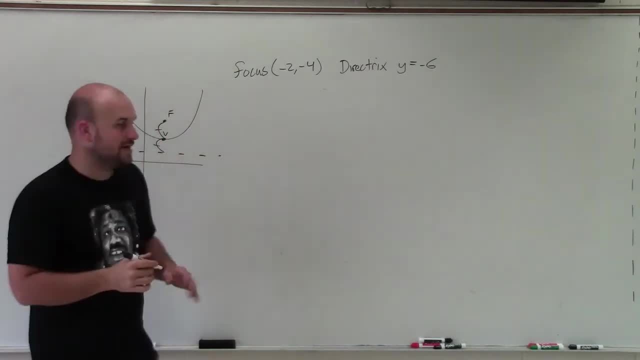 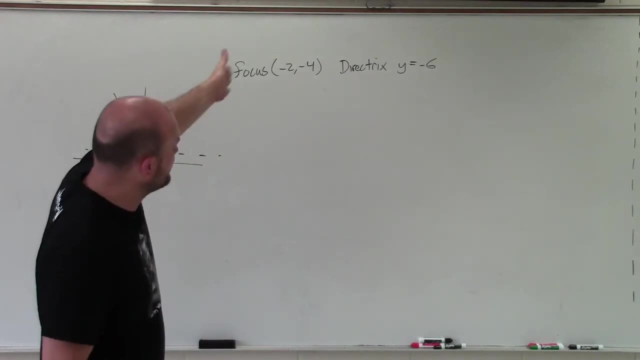 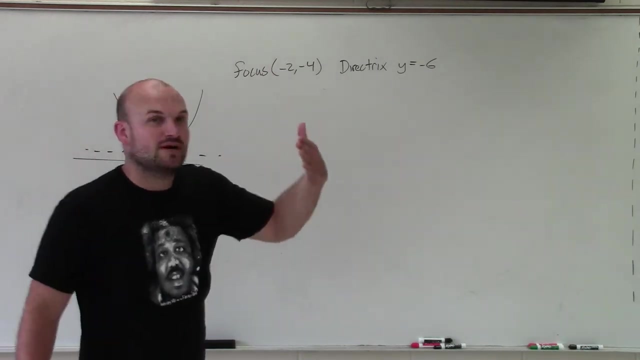 from there to there is going to be equal, as that represents the directrix. So what I want to do is I'm going to want to plot both of these. I'm going to want to plot the focus and as well as determine the directrix and see if I can determine where the vertex. 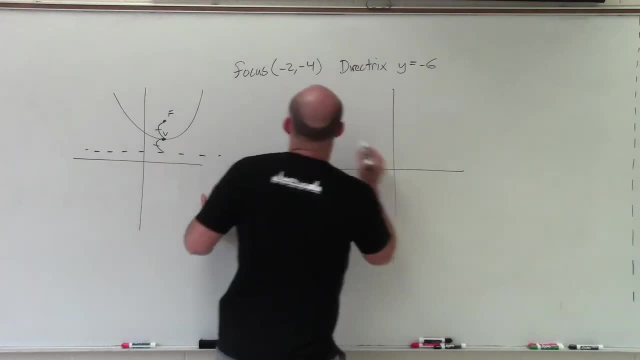 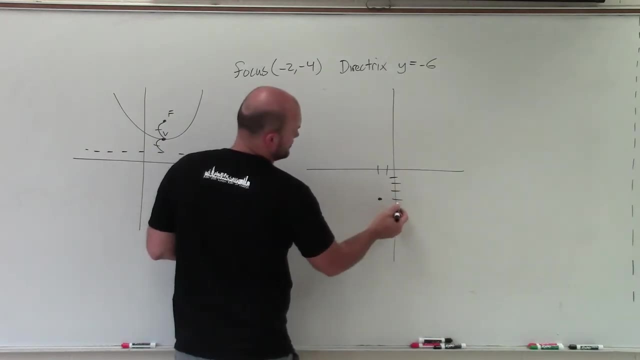 would be. So let's go ahead and plot this information So I have. the focus is at negative: 2.. Negative 4, 1,, 2, 3, 4.. And the directrix is at y equals negative 6.. So 4, 5, 6.. OK. 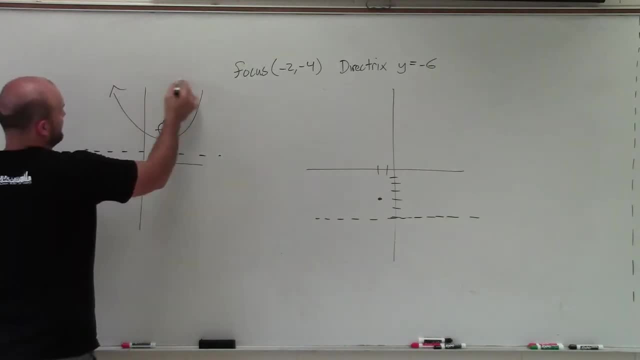 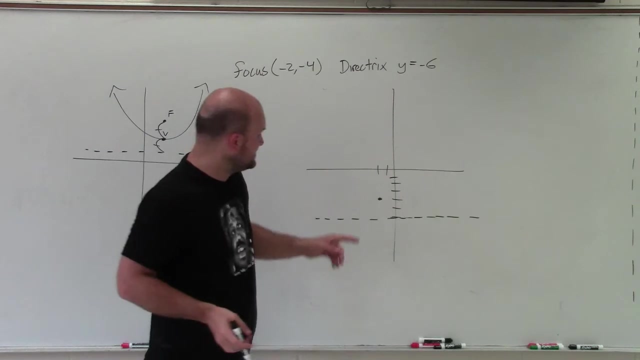 So remember looking at our parent graph here of just any parabola, we notice that the direct focus is inside of the parabola, right. The parabola goes away from my directrix. So if here's my focus, that means my parabola has to be half the distance between the focus. 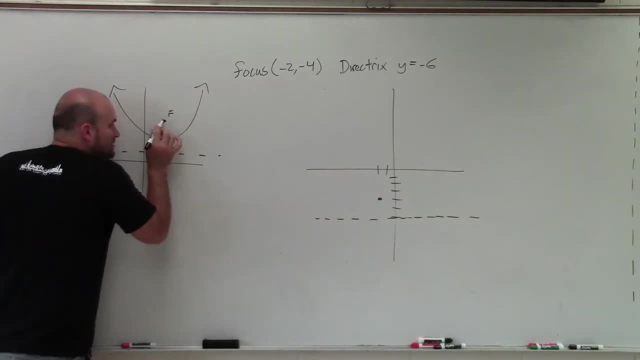 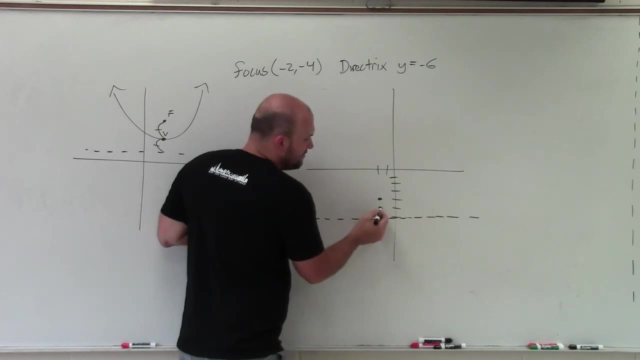 and the directrix right, Because, remember, the vertex is equal distance to the foci as it is to the directrix. Well, since there's only two units between these two, my focus has to be at this coordinate. I'm sorry, My vertex has to be at this coordinate And there's 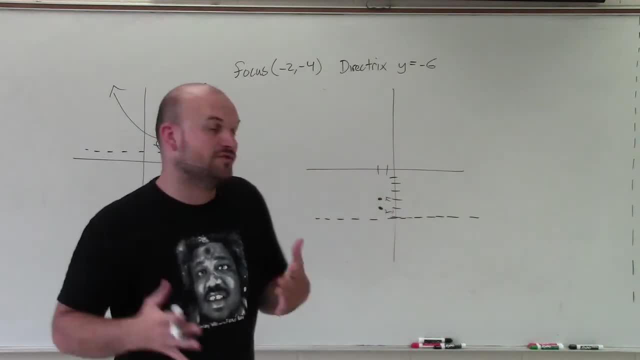 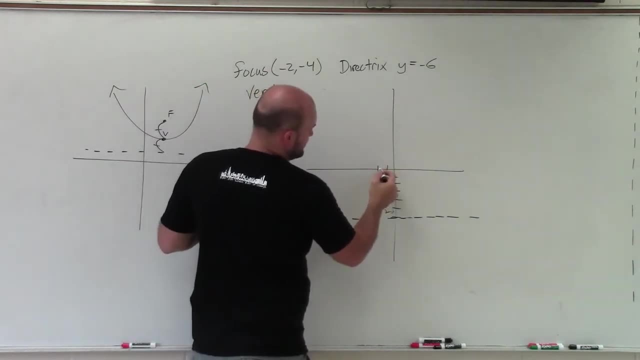 my focus. Now, why is it so important to find the vertex? Well, one to write the equation. we want to know what the vertex is, And the vertex in this case would be negative 2, negative 5.. 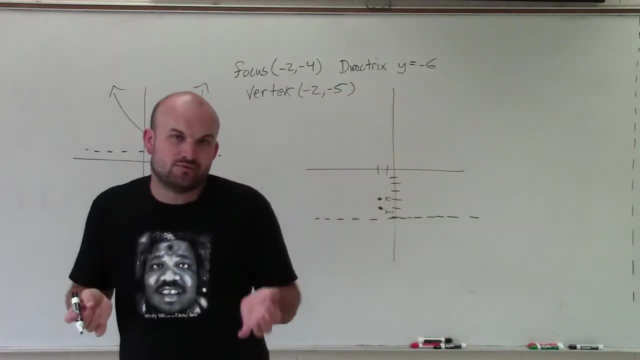 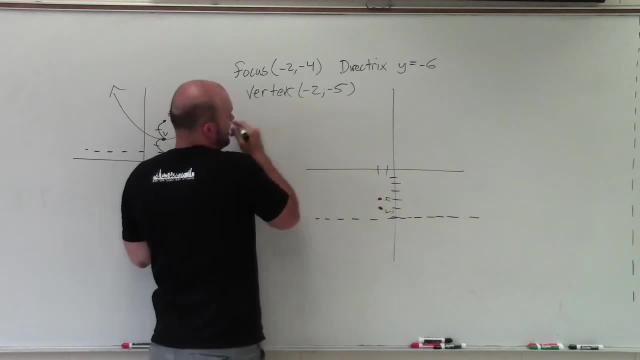 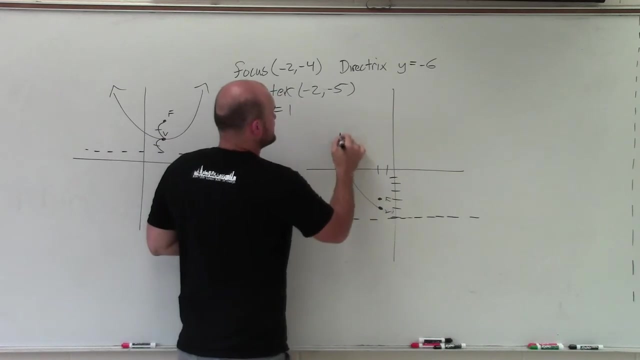 Also, to write the equation, we need to know p, which is the distance from the vertex to the focus. Well, since my vertex to the focus is going up, I can say that's my vertex to my focus. I can say p is equal to 1.. Now, since I have x squared, I know I can use the.